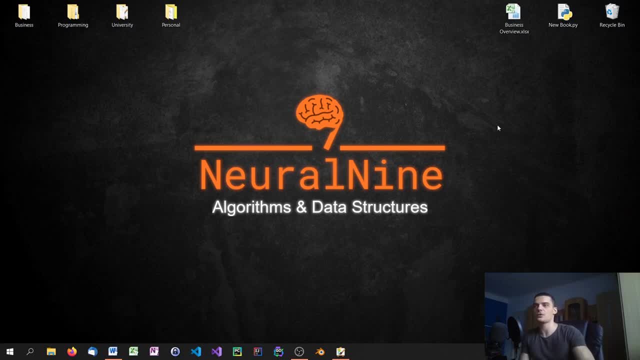 save these big data sets on and also these external storage media usually have a block-oriented structure, which means that when you access one thing, you access the full block, not just one individual element, but you access the full block, and because of that it makes sense to come up with 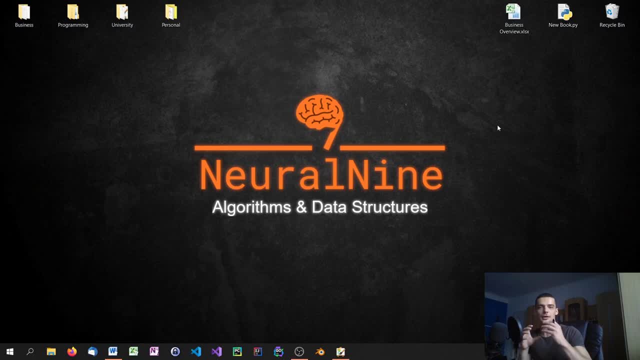 a kind of tree structure that allows you to save these big sets of data. It allows you to store information in blocks and thus limit the height of the tree, because when you limit the height of the tree and you can still do all the operations in logarithmic time, it's not only logarithmic runtime complexity, which is already very good, but you also have a very, very small height, which means that the logarithmic, or the logarithm of the elements, is actually very small. so you don't only have a very efficient runtime complexity, but you also have very few levels that you can navigate to, and this is a very 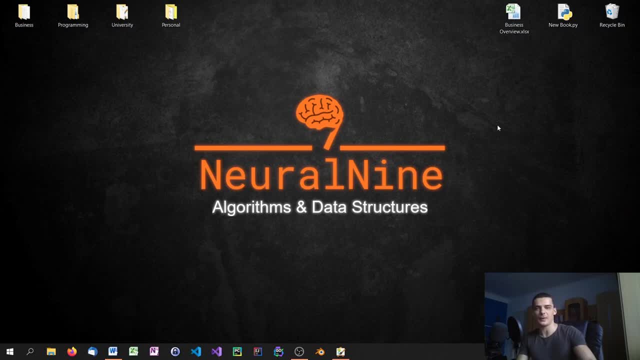 good thing, because because of that, we limit the amount that we have, the amount of times that we have to access data or we have to to ask left or right, for example, or left, right or middle, for example. so this is what we're going to do today: we're going to talk about b-trees, so let us get right into it. 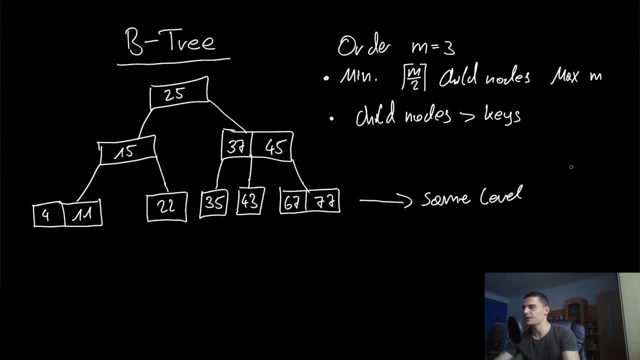 so now let us look at this example of a b-tree. here we're not going to talk about the formal definitions, the exact formal definitions too much. we're just going to take a look at what a b-tree has to be kind of, and then we're going to talk about how to rebalance it, how to 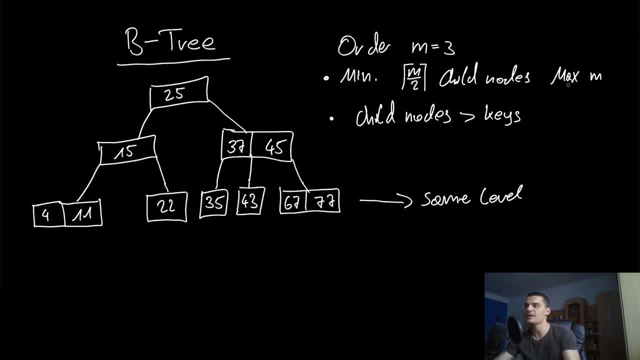 insert elements, find elements and so on. now every b-tree has a certain order and this order in this case is three. so m is the variable for the order. in this case, we have a b-tree of order three and this means that we can have a maximum of m child nodes. now, in this case, you can see: 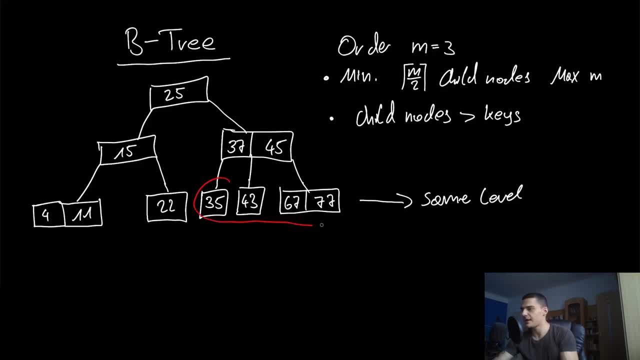 of three child nodes. sorry, in this case you can see here we have three child nodes we have. so this thing here is one node, one block, and this one block here can have three children as a maximum, but at the same time it has to have m divided by two and the result sealed, so rounded. 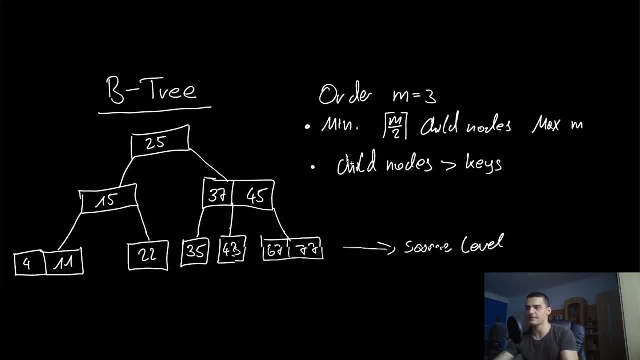 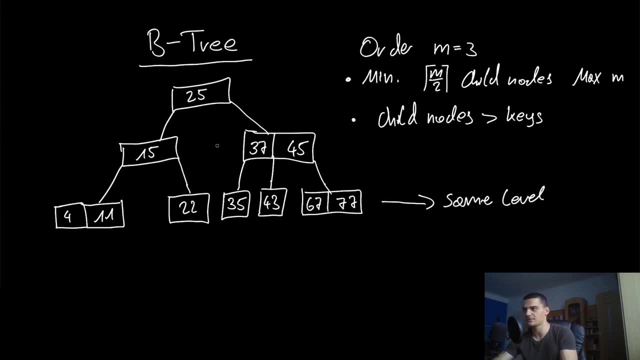 up, uh, child nodes as a minimum. so except for the root node, example, uh, for example, the root node has to have a minimum of two children. the root node has to have a minimum of two children. but all the other nodes, except for the leaf nodes of course, um have to be. i have to have a minimum of. 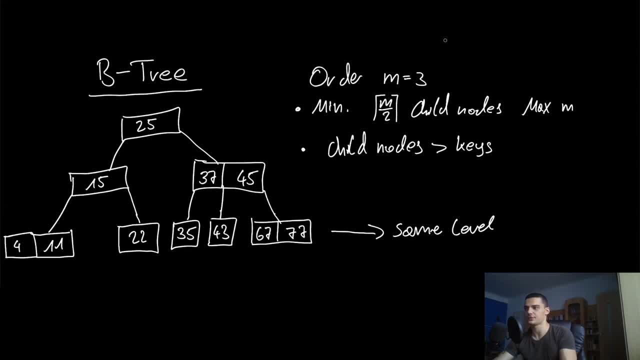 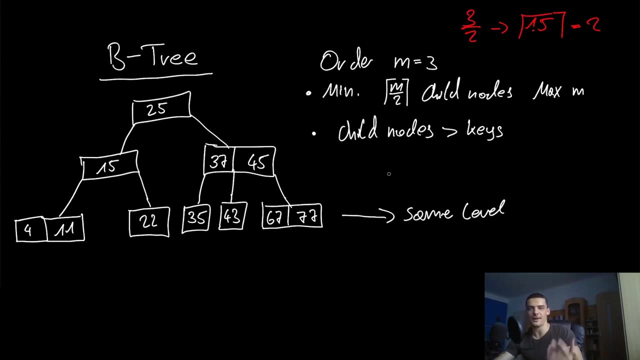 m divided by two, and the result sealed child nodes, in this case three divided by two is 1.5, and 1.5 sealed is two. so we'd have a minimum of two child nodes. um, what does that mean? this means that if we are below the minimum or above the maximum, we have to open up a new level. 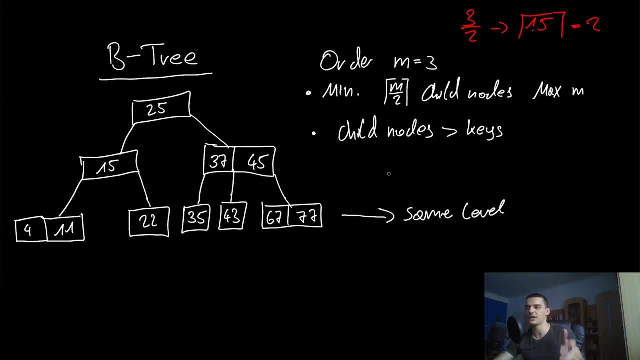 we have to reship values, we have to rebalance the tree, adjust the structure so that we can fulfill this property. also, the amount of child nodes has always to be larger than the amount of keys. so if i have two keys here, i have three child nodes. if i have one key, i have two child nodes. if i would have a b tree of order, six or 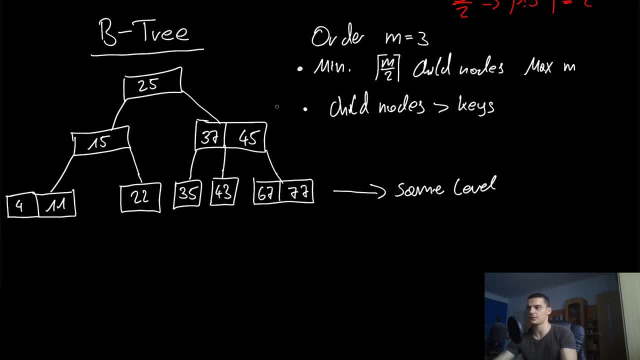 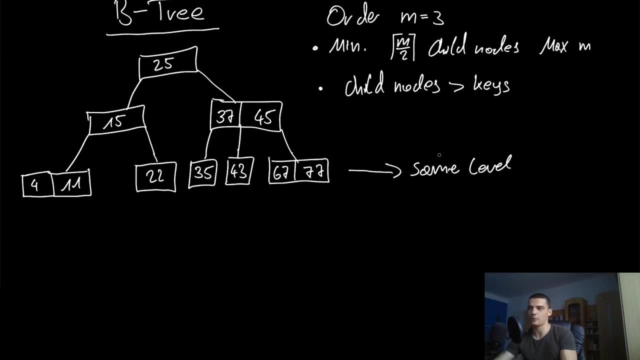 something and i have five keys, i would have to have six child nodes and so on. so this is another rule that has to be fulfilled when we're talking about b trees. and one rule that's also very important is: all the leaf nodes are at the same level. the leaf nodes are at the same level, which 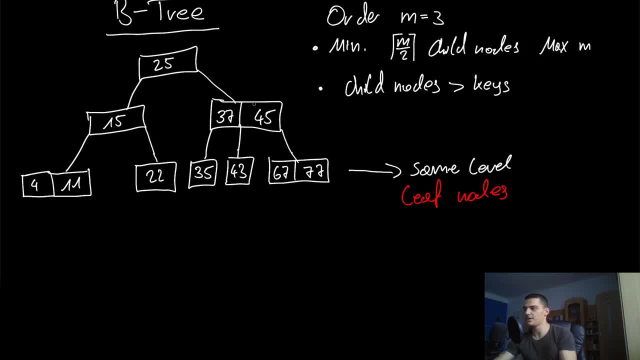 means that we cannot have um a bunch of them here. and then you know, i mean, it doesn't make sense anyway now. but i cannot just go ahead and open up this here as a new level. and then i have some leaf trees here, um leaf nodes, sorry leaf nodes here, and then some leaf nodes here. all the leaf nodes have to be at. 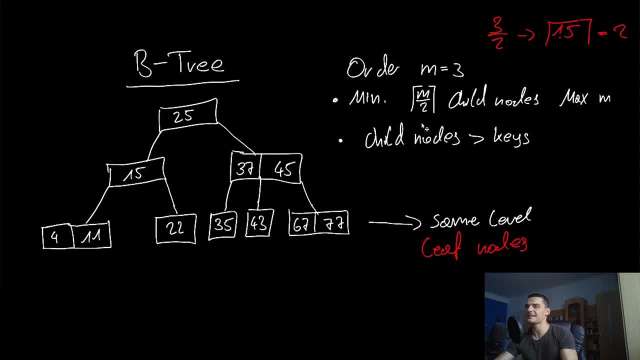 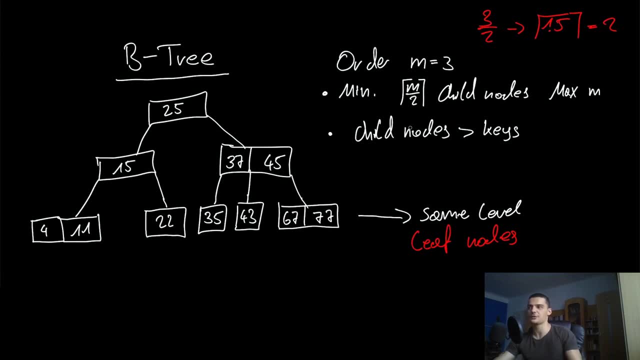 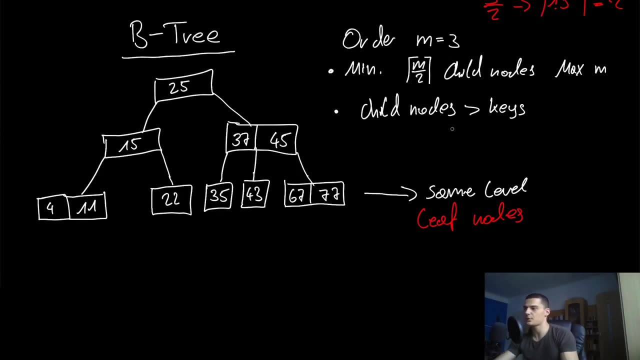 the same height at the same level, and those are basically the criteria for a b tree, and once these criteria, or as soon as these criteria are not fulfilled anymore, we need to rebalance, restructure and do something about it. so let's go ahead and try to insert a new element and unbalance the 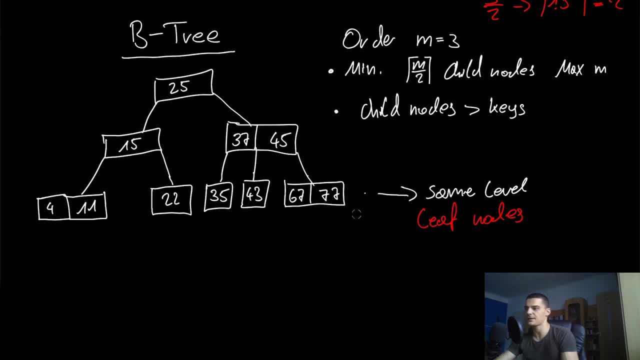 b tree or violate these criteria, to see what happens. now let me just delete this real quick, and what we're trying to do now is we're going to add the element 80 to the b tree and see what happens and see how we can rebalance it. now, if you want to add the element 80, i go to the root. 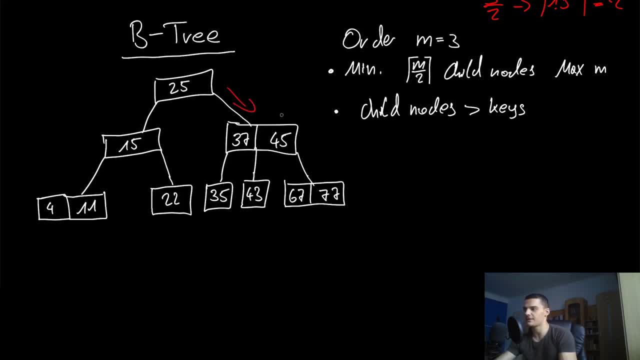 node. it's 25, so i need to go to the right. then we have 37, 44, uh, 45. sorry, 80 is larger than 37, so we're not going to the left. it's also not in between 37 and 45, because then we would have to. 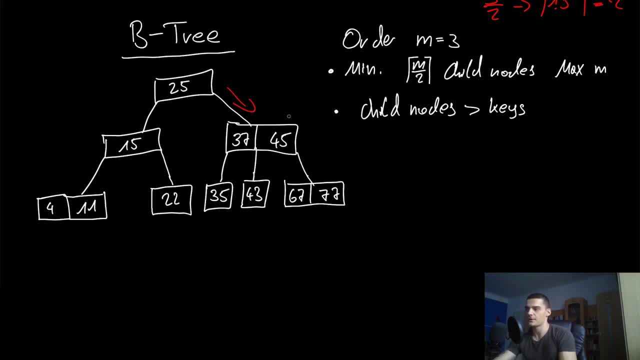 go down here. that's not the case. so we're going to add the element 80 to the b tree and see what happens. uh, but it's larger than 45, so we need to go to the right, and then we have those two keys here, so we have 67, 77 and um. actually would have to go to the right, but since we're at the leaf level, 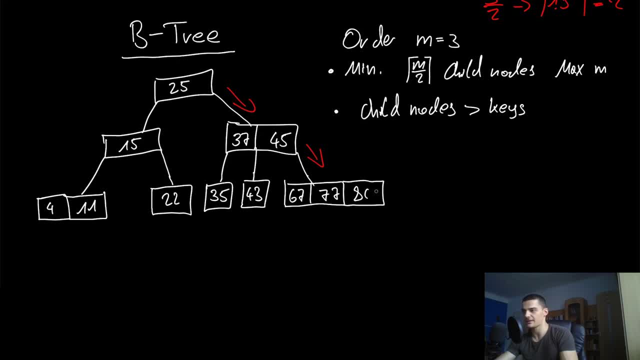 we just append it here into the same block and see what happens now. the problem is that we have a block of three with three keys, which is not allowed because we have the order three, which means that the maximum amount of keys is two, because the child nodes has always, uh always. 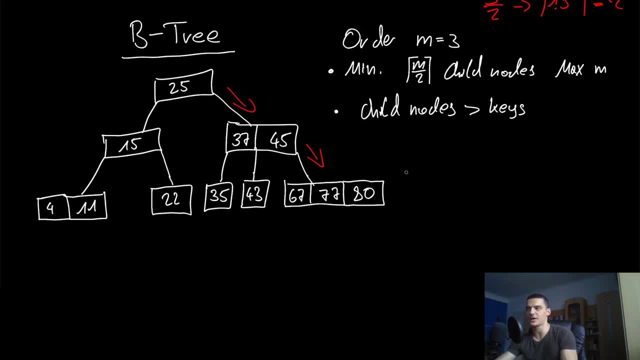 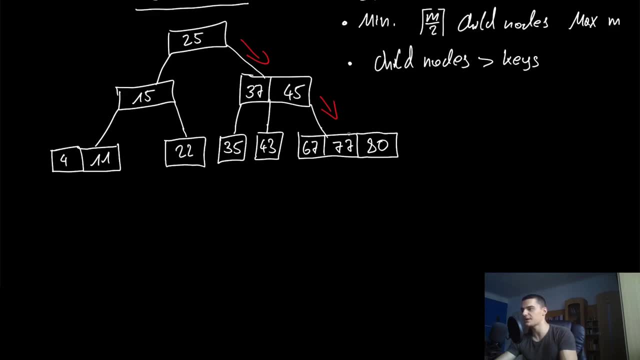 have to be larger than the keys, and the keys cannot be larger than two if the child nodes have a maximum of three or are a maximum of three. so what we need to do now is we need to adjust. so what we do is we uh shift up the center value one level. uh, shift it up one level. 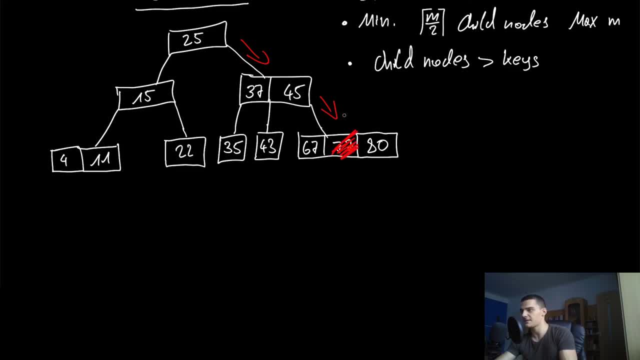 yes. so what we do is we essentially say by 77, and we shift it up, uh, into this level here. so actually, let me just delete a bunch of things here so that it doesn't look too messy. we just delete this, uh. so actually 77 is the maximum amount of keys, so we're going to go to the left and we're going to 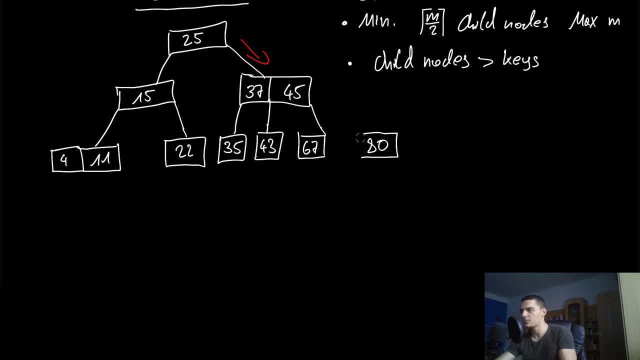 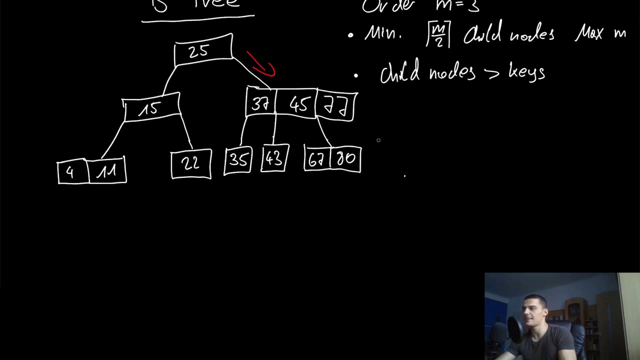 remove it from this leaf level here, and what we would do next is i'm also going to delete the 80 here and rewrite it. so now we have 80 down here and we have 77 up here, uh, but now we have the same problem here because, um, here we also have three keys and, of course, you know what i could. 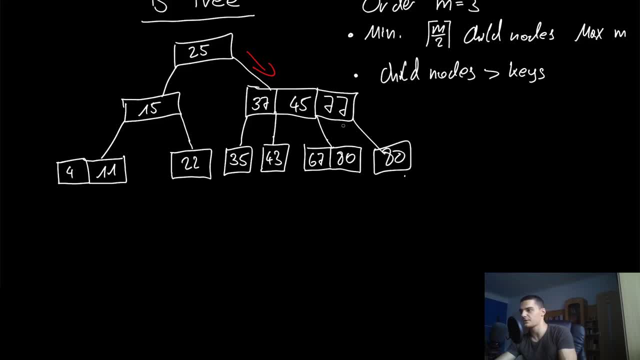 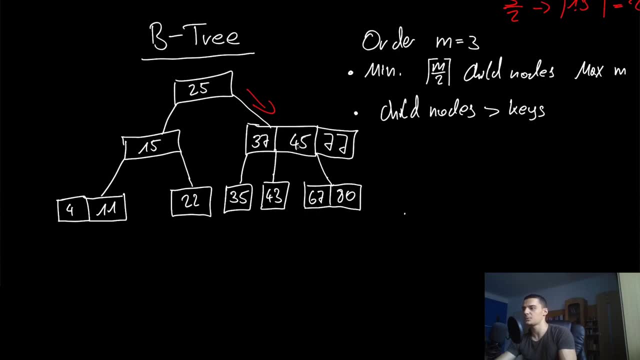 do is i could say: okay, then we have 80 because obviously we need to do it like that or something, but that doesn't make sense because we are not going to leave 77 here because we have a b3 of order three. so what we do here next is we shift up the center value again, and what happens? 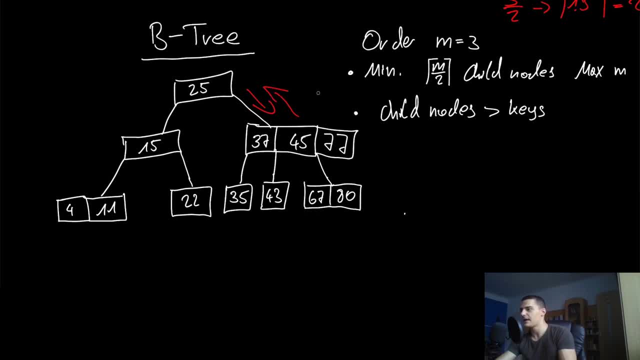 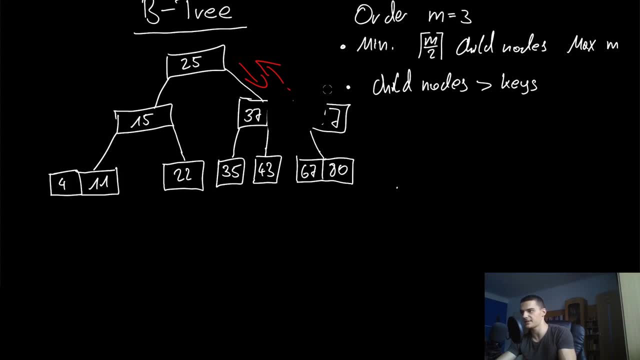 then is we shift up 45 into the root node, um, and then essentially what happens is we remove it and we essentially replace it by 77. we replace the position by 77 with 77, and i'm not sure what number. it was 45. uh, i think it was 45. 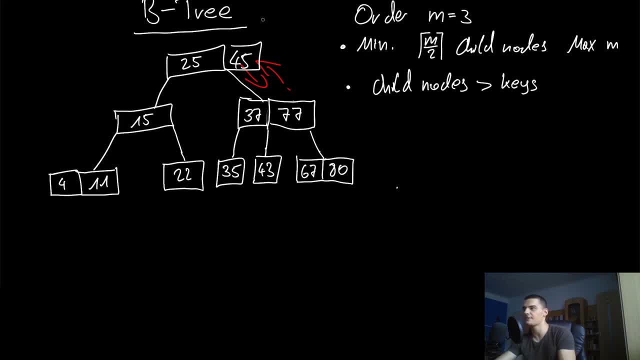 we end up with this here, and because we end up with this here, we have two keys and three child nodes. we cannot just have two child nodes and two keys. we need to, um, say, the middle points to 37 and the right points to 77. so let me maybe again clear this up a little bit here, so that we don't 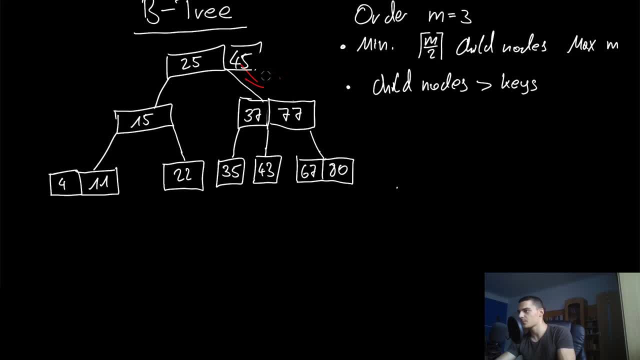 have it too messy, um, we're just going to delete these red arrows here and redraw the 45. so what we would do is we would say: okay, these are now separate blocks, so again, we're going to split them like that and we have 37 here and 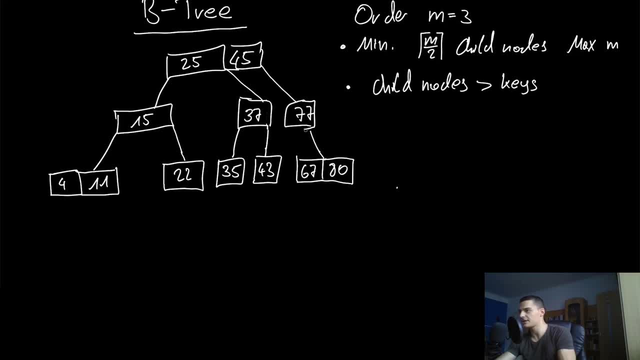 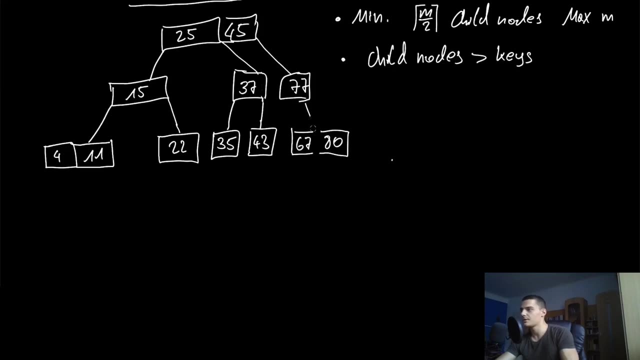 77 here, and then we connect those two and then we say, okay, to the right, you have 80, to the right, to the left, you have 67. so essentially you also split these two nodes here. come on, don't do any dumb shit here. we have 80 here. 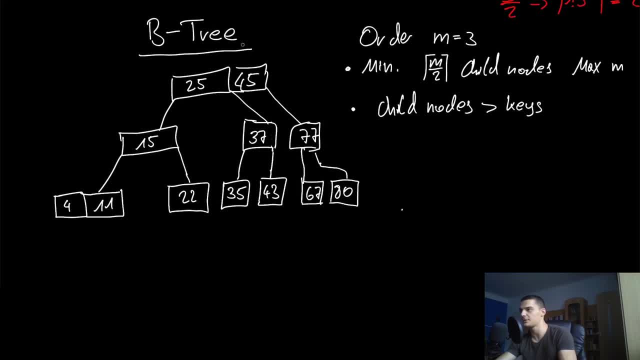 and 67 to the left. it's not the most beautiful tree that you can draw, but that's essentially what you do when you enter an element and the structure uh violates the criteria. shift up the center element because we had three keys at the leaf level, so we shifted up the center key. 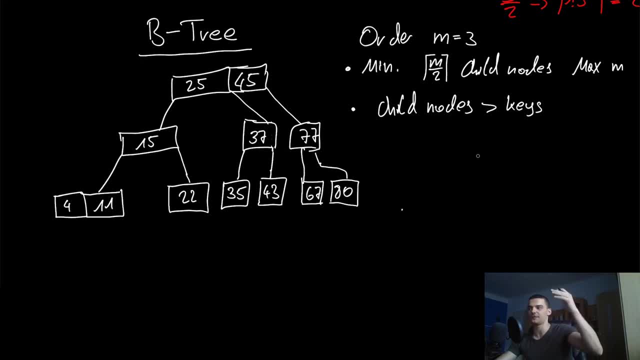 then we had three keys at one level above that we had to shift the center key again and now everything's fine because we have two keys. that's okay. in a b tree of order three, we have a balanced structure here. we can find elements in logarithmic runtime complexity. it's not going to work between 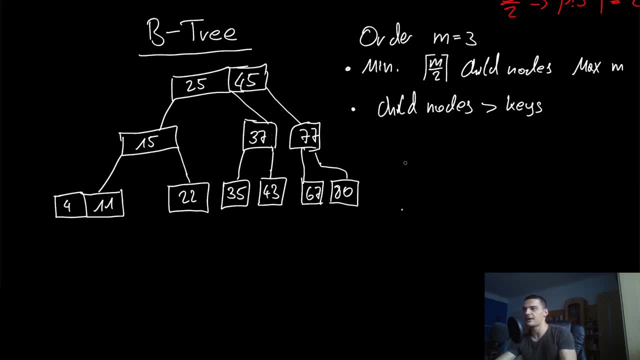 all the fours in one tree and then we can split them by a teaspoon or so that these three keysud 뭘, something on the indicate, mean that we can't choose anything off wall loop. that would obviously mean it's not a problem and all these um criteria are still satisfied and met. remember we had the leaf. 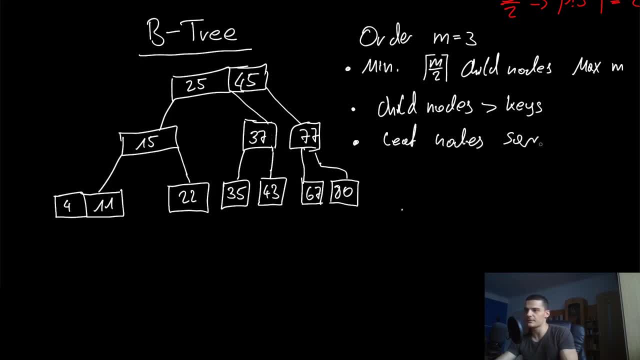 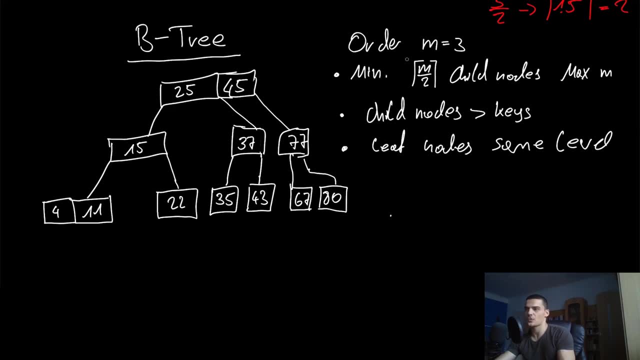 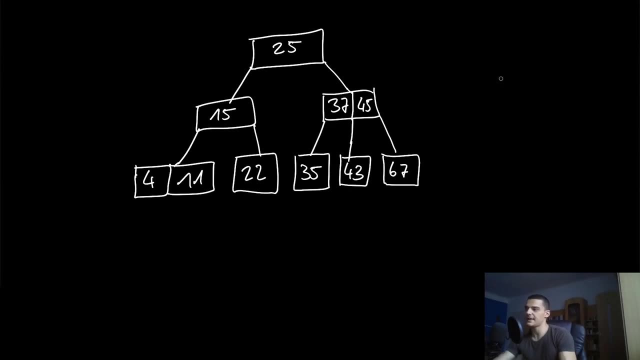 nodes, leaf nodes same level, leaf notes had to be at the same level level. uh, and all these, um, all this criteria here is satisfied, so the b tree is rebalanced. now let's look at what happens when we delete elements and violate the criteria. what happens then is: uh, i mean, it depends on what kind. 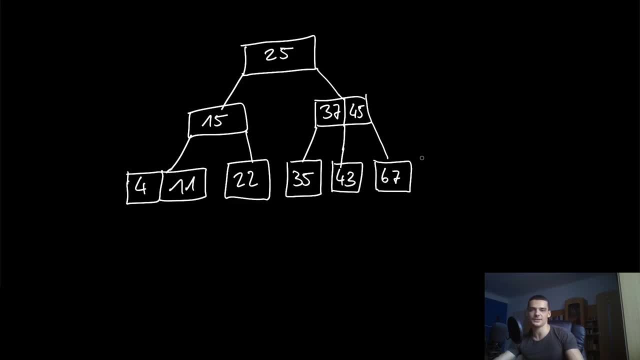 of deletion you perform, because in btrees you have many different scenarios for insertion and deletion. my recommendation to you is, if you want to get a basic understanding of what's happening- or not a basic, but a deep understanding of what's happening- i would recommend going online and 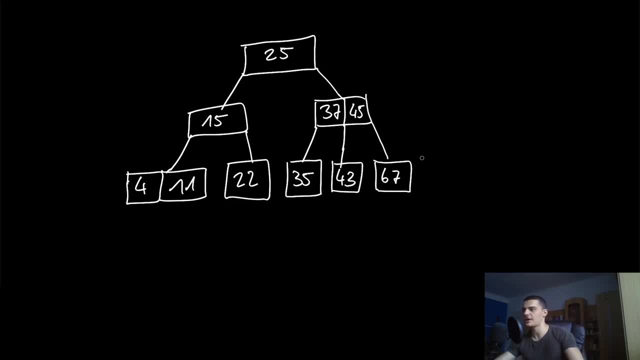 typing btree simulator into google or duckduckgo, whatever, and play around with it a little bit, because reading the formal definitions, you know you can learn it. you can memorize everything, but i think it's really important to have a good understanding of what's going on and how you're 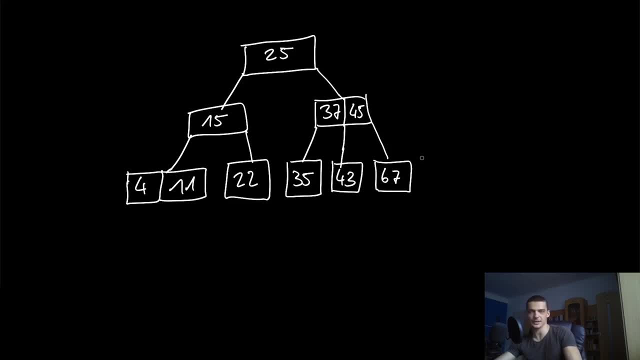 going to use it and how you're going to use it and how you're going to use it and how you're going to. you'll get more of an intuition by playing around with a simulator, with a visualization tool. you can also, additionally, go to a textbook and read all these definitions there, but i think 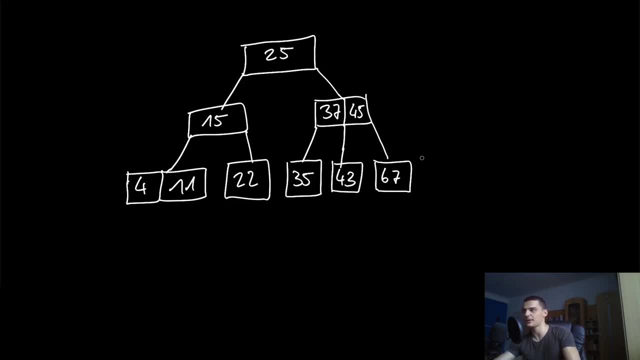 they're going to confuse you more than just playing around with the simulator. but essentially you know, if you delete a read, if you delete a leaf node, what happens is you essentially just rotate so that the missing place gets filled up. so in this case, if we delete 22, for example, 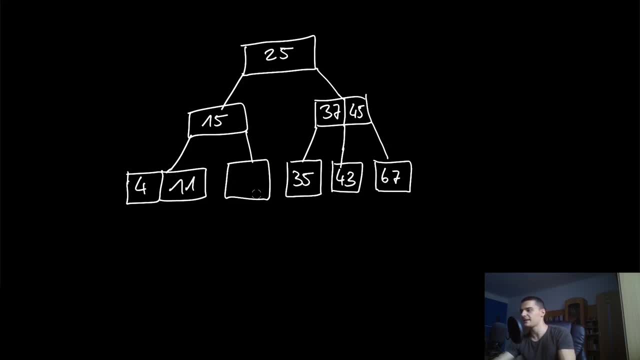 what would happen is we would of course delete 22, and then the obvious thing to do here is you just have to rotate so that 15 ends up at that position here and you shift 11. so you shift 11 up here and 15 down here and you'll rotate basically in a similar way to, uh, the avl tree rotation, so that 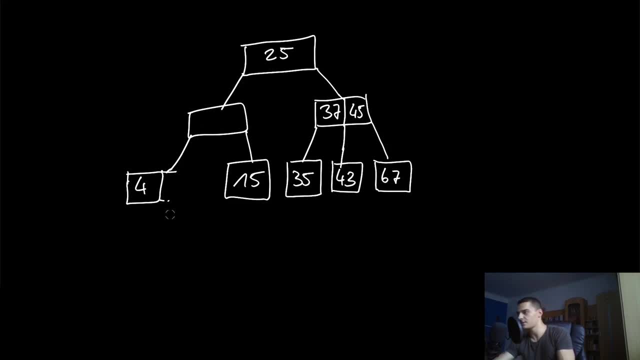 you end up with four at the left side and 15 on the right side and in general it's 11 up here. so that's a single rotation, a very simple rotation. if we delete a re, if you delete a leaf node, now what happens when we delete a node in between and a level in between? uh, this is a little bit. 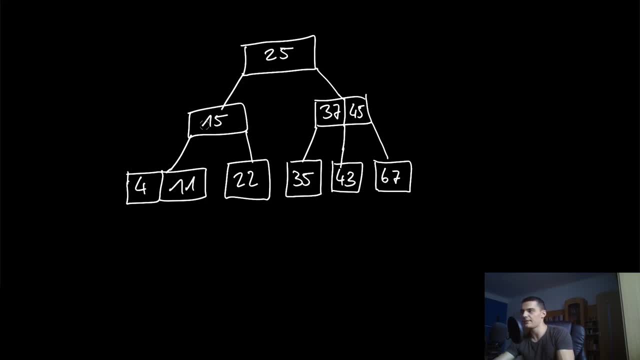 more complicated, but it's still very similar to the avl rotation. so if we delete 15, for example, what happens now is we rotate the whole tree. so we say this is a rotation here, and what happens is we have 25 here now um, and we replace 25 by 37, but then we need an additional um, so we say 37. 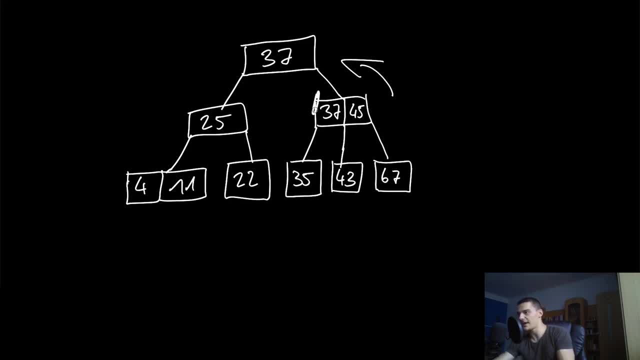 but then of course we need an additional rotation here, because now we have- uh, we have- this node here removed and we have only one key at this level on the right side, and because of that, of course, we cannot have three children here. but it would also not be correct to just take 35 and put it. 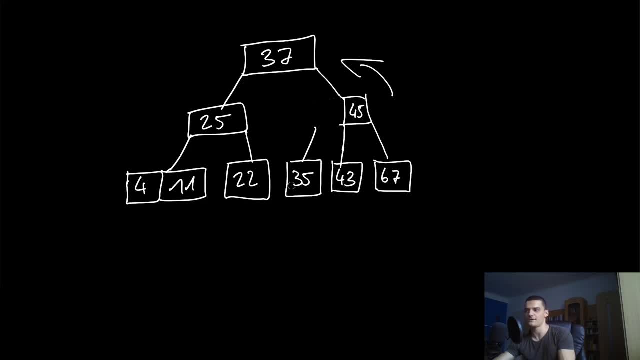 into the same block as 43, because 35 is actually less than 37 and cannot be on the right side. so what we do is we actually combine these two blocks here, so actually 35 and 22 are combined. so 35 and 22 are combined, and that's how you rebalance the tree, in an avl like way. so you 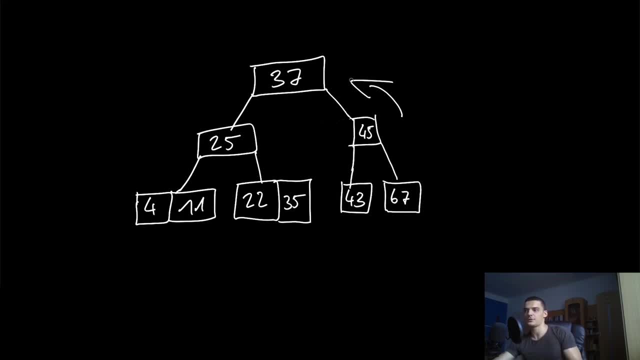 essentially just rotate the way, uh, that you need to rotate in order to fill up the empty slots, and then you um make sure that the individual elements are on the right side, uh, like, not on the right side, but on the correct side, um, and, as i said, if you want to get a real good feeling about this, 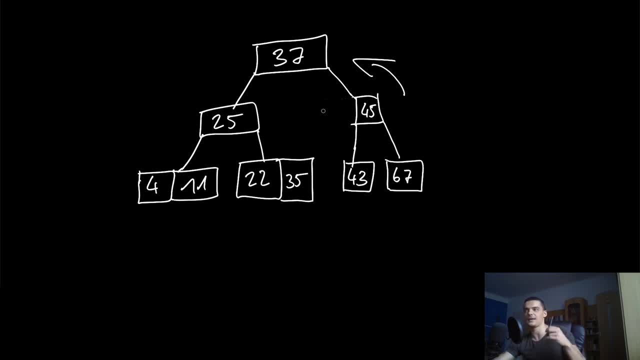 a really good intuition about this. i would recommend playing around with a visualization tool. uh, there are a lot of visualization tools for b trees online. uh, because, as i said, i don't see a lot of value in reading the exact definitions unless you want to program an algorithm with it, or 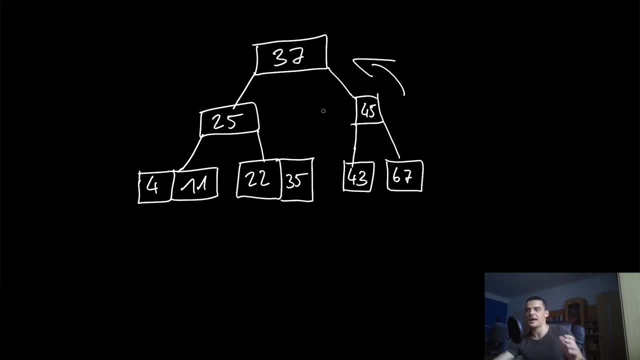 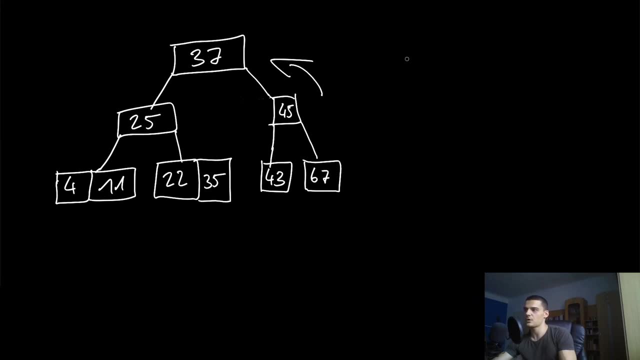 something like that. but in order to understand what b trees actually does and how they balance them, rebalance themselves and so on, i think it's enough to just play around with the simulation tool. now, last but not least, we're going to talk about why this is possible in logarithmic time. 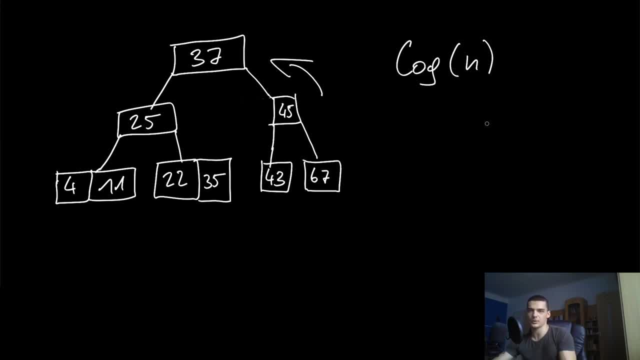 again, uh, obviously, because the rotations, in the same way that it was true for the avl trees, we're not going to have more rotations than there are levels, um, or at least not single significantly more. so we'll end up with logarithmic runtime complexity. and also, when we have uh, when we add. 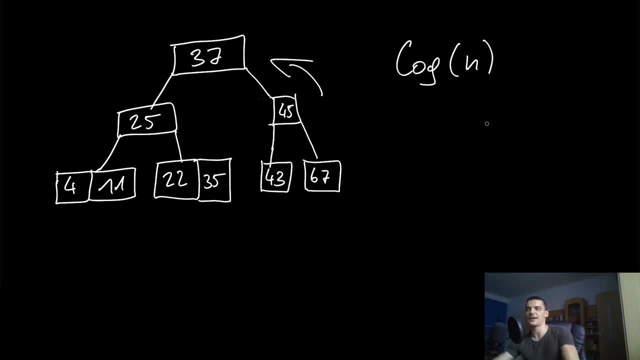 elements. we need to shift up, shift up, shift up and so on, but we cannot shift up more times than their levels because then of course we would be above the root node and this doesn't make sense. so all these operations- finding elements, adding elements, inserting elements, removing elements or rebalancing the tree- everything is possible in 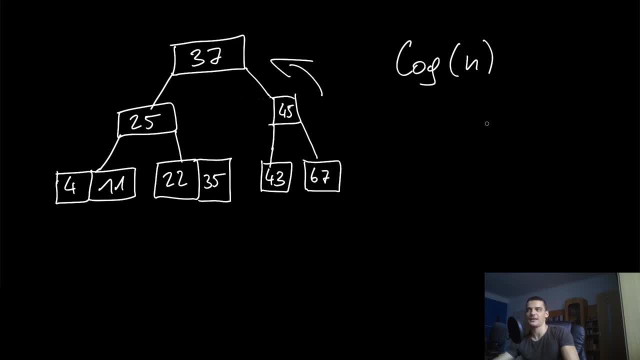 logarithmic time. but b trees have the additional advantage that we have data saved in blocks and because we have more data in one node, in one block, we have less, less many times, we need to access less many times, and this is very beneficial when it comes to external storage media with 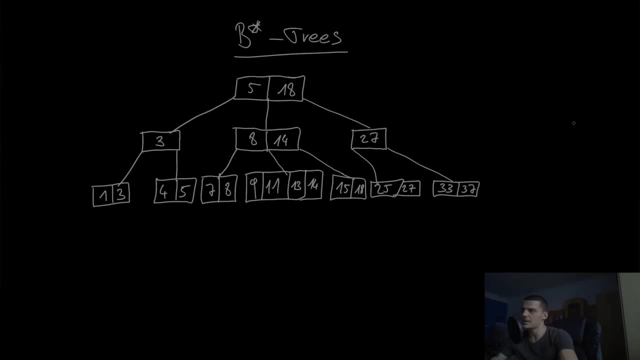 a block like structure or block oriented structure. so last but not least, we're going to talk about b star trees, which are a little bit special because all the nodes in between here, all the values in between here, are just used for navigation. now the b star tree has the property that all its elements 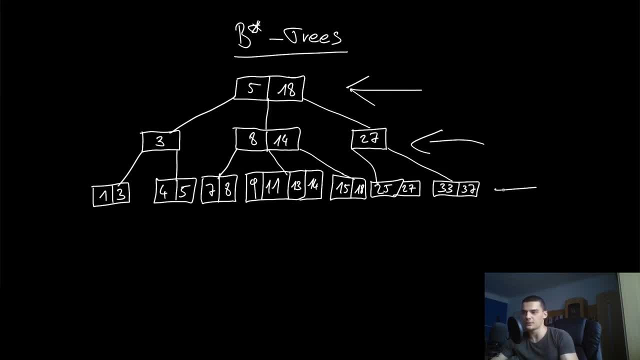 all its actual values that we're interested in are leaf nodes. we don't have any value that we're interested in that is not a leaf node. all these values here are just values that are guiding us, that are navigating us towards these values that we're actually interested in. so 3, 8, 14, 27 are just. 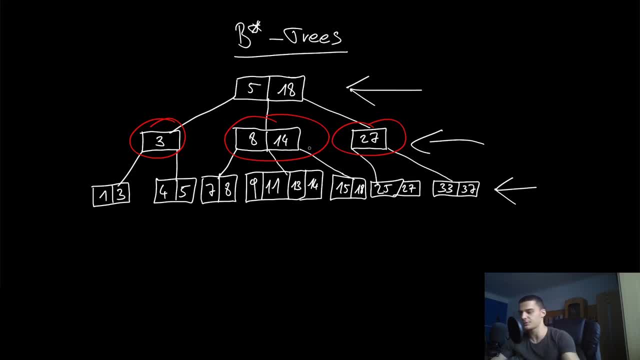 values to tell us you need to go left, you need to go right, you need to go to the center and so on. now, this is essentially what a b star tree is, and this number- here the value of the navigation key- is always the largest element of its left child. so in this case, you know. 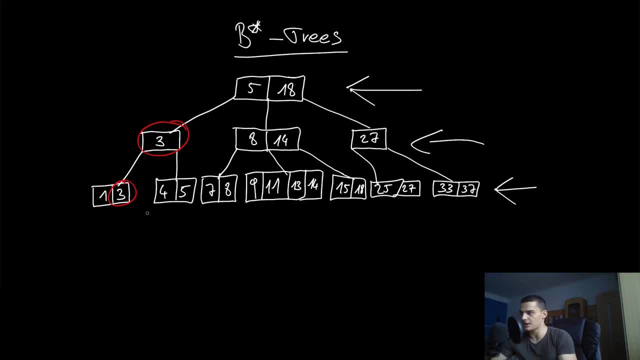 you have 3 because 3 is the largest element of its left child tree, the actual element. we're not talking about navigation elements. 5 is 5 because it's the largest element of this left subtree. 8 is 8 because it's the largest element of the left subtree. 14 is 14 because it's the largest element. 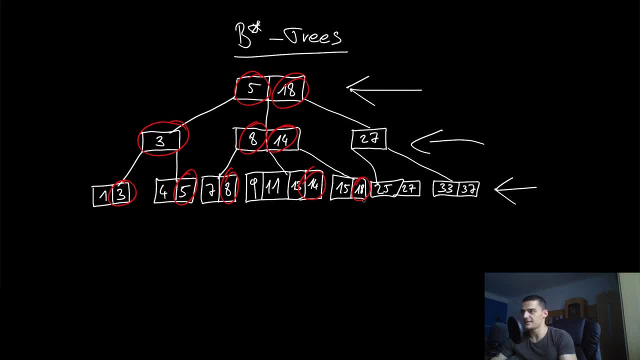 of its left subtree, 18 because 18, left subtree, 27 because 27, and so on. So it's always like that and this is the pattern here. We always have these in-between layers in order to navigate and the amount of, actually the amount of elements that we can store at the leaf level is determined. 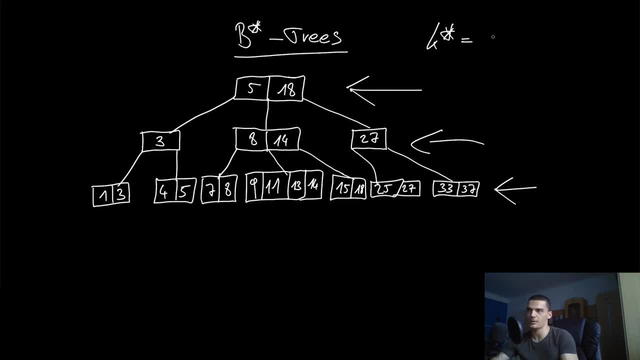 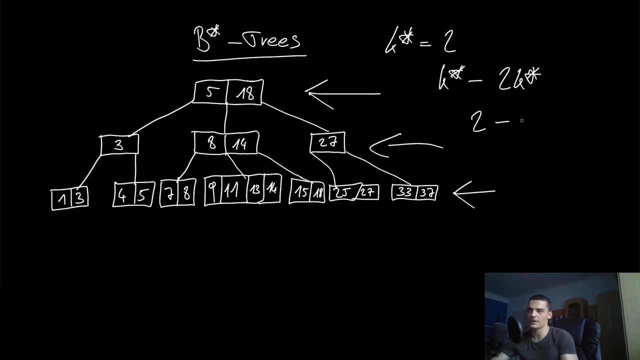 by a so-called k star parameter. In this k star parameter- let's say it's two- in this case means we can have from k star up until two k star elements at the leaf level. So you can have a minimum of two or a maximum of four. So two, three or four elements at the last leaf level. 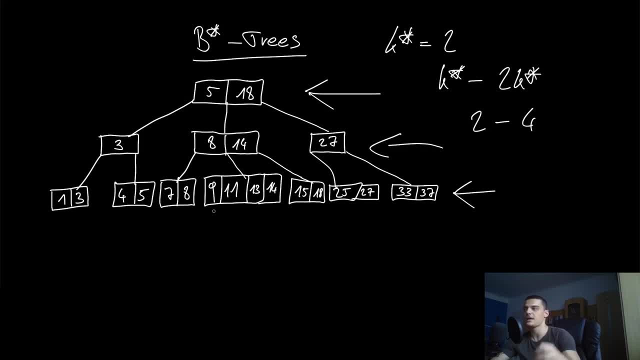 You cannot have less than those. You cannot have more than those, because if you have more or less, we're going to restructure the whole tree. We're going to add an additional level or we're going to remove a level and restructure everything so that it still fulfills this criteria. Notice, however, that 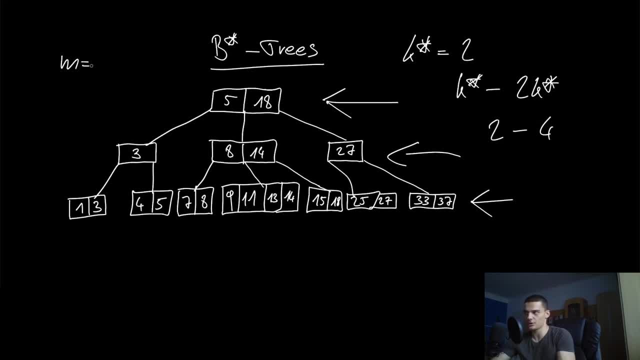 this parameter here is different from the m parameter from the order of the tree. The order of the tree is still three here, so it's an ordinary b tree, but we have the property that in the leaf level we can store two to four elements per node. So this is essentially what a b tree is. 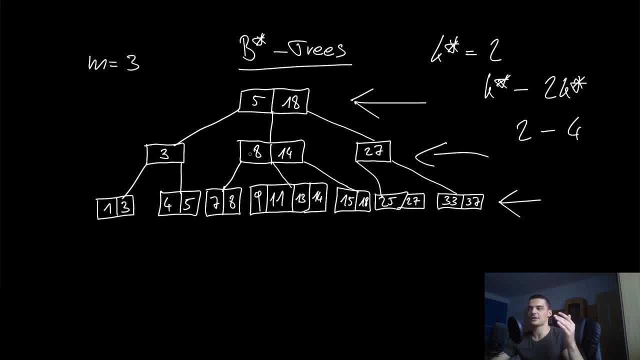 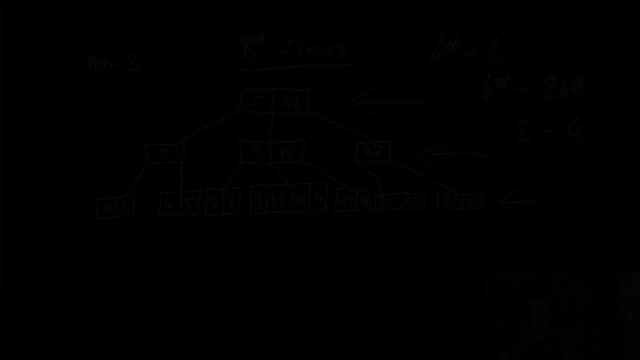 a b star tree is a b tree where we have essentially all the layers In between are just used for navigation and all the actual data is stored at the last level, at the leaf node level. So that's it for today's video. We now talked about b trees and b star trees- B star. 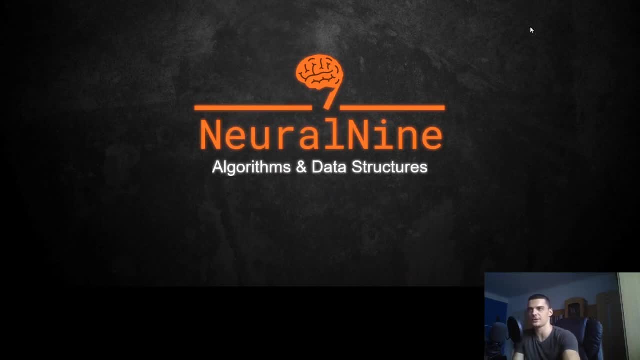 trees usually have a smaller height than b trees because you know you only need the navigation tools and all the data is stored in large blocks at the leaf level. So you have a smaller size, a smaller height of the tree And you know. for now we're done with the algorithms and data structures. 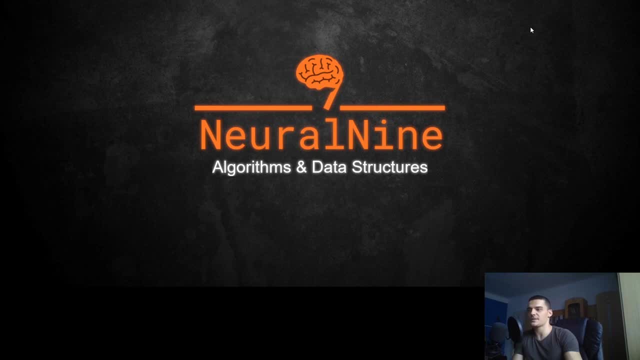 tutorial series for beginner, for beginners. We have a lot more topics that we could cover here, But I want to focus more again on Python projects, on AI projects. It was a an interesting tutorial series and I know that a lot of you enjoyed it and it was very popular in the 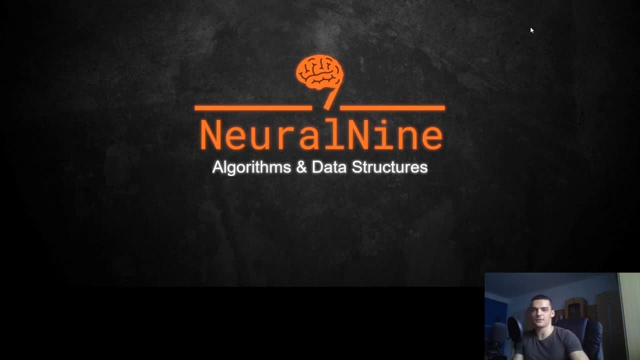 beginning, The more advanced topic got less views because probably they're either too complex or not too interesting to a lot of you guys. If there is enough demand and if I notice that there is interest in more advanced topics like p problems and p problems and p complete problems, all these dynamic programming, 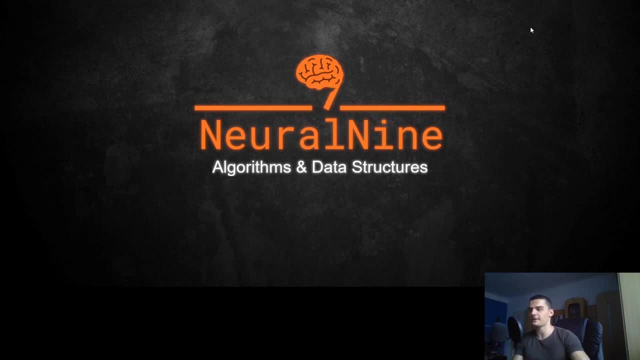 issues and so on. If there is demand for that and if I see that people are interested in it, I might make some more videos, But for now, this algorithms and data structures tutorial series for beginners is done. If you have any questions, you can leave them in a comment section down below, If you like this. 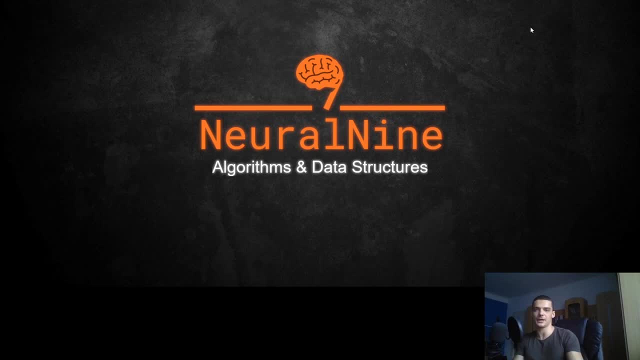 video or the whole series. you can leave a like and let me know in a comment section by writing a comment about that. Also, make sure you subscribe to this channel in order to see more future videos for free. We're going to do a lot more Python now again. a lot more projects, a lot more. 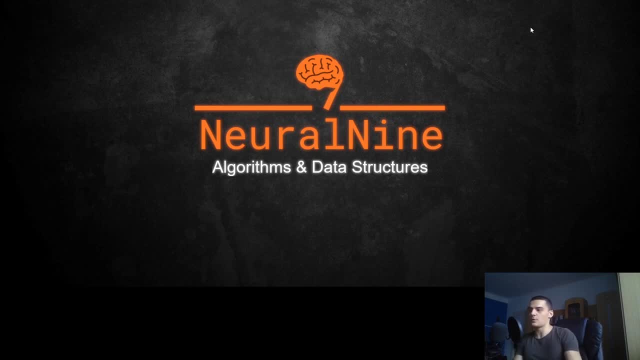 networking, AI and so on. So we're going to get back to you, To the old kind of videos here. So thank you very much for watching, See you in the next video and bye.